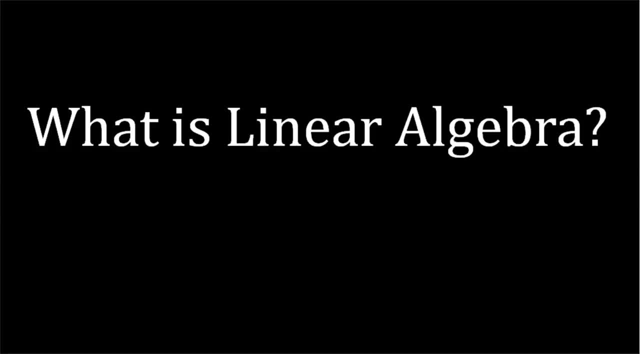 All right, hi everyone, and welcome to our first video in linear algebra. We're going to start by trying to answer a very basic question: what is linear algebra? Now, I know, of course, we can't give a completely comprehensive answer, but maybe we can come up with one that's enough to get us. 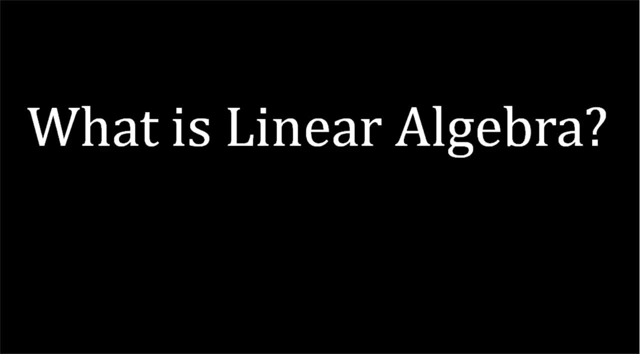 started. Something like trigonometry is the study of triangles, or calculus is the study of rates of change. Just something very basic like that that'll help us frame the course, maybe, and get ready for what's coming. So one of my first instincts when trying to come up with an 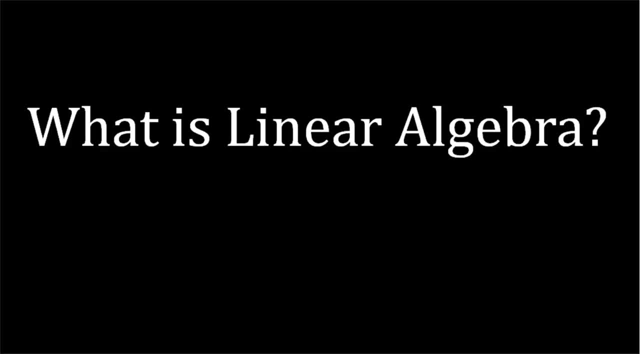 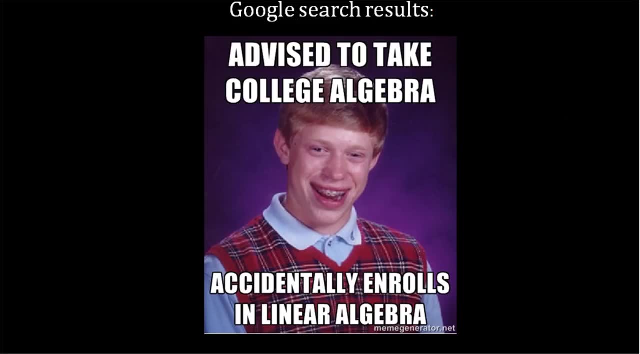 accessible answer to this question is probably very similar to your first instinct. I googled it and one of the first things I came across was this linear algebra meme- of which there are many, which I found really surprising. But anyway, next I went to: 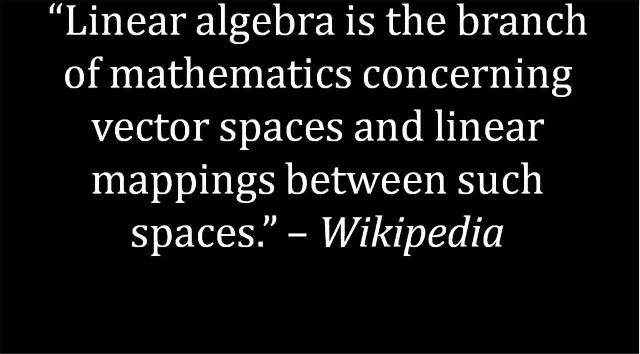 Wikipedia. Wikipedia says that linear algebra is the branch of mathematics concerning vector spaces and linear mappings between such spaces. Now let's all take a moment to digest that. Okay. so here's the thing with this definition. it is impeccably accurate, impeccably correct, But the problem, at least for our purposes, is that it is not at all. 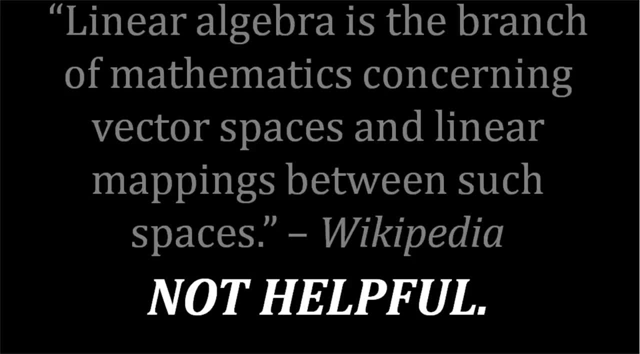 helpful. Can you imagine telling somebody who does not know anything about linear algebra that linear algebra is the branch of mathematics concerning vector spaces and linear mappings? The truth is that if you know what those things are, then you already know what linear algebra is, So I'm not a big fan of this definition. 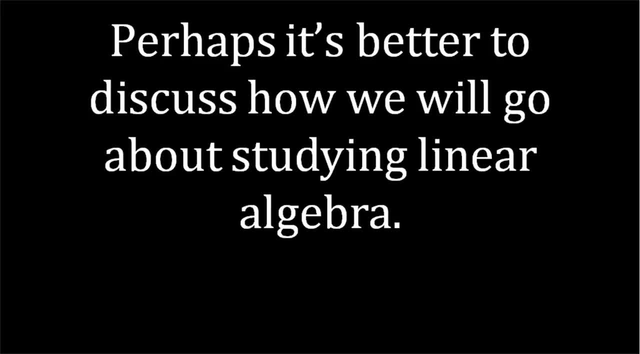 So we are going to try to answer this question a little bit differently. We are going to discuss how we're going to go about studying linear algebra. In other words, there are many different pathways in the algebra and linear logic into this subject. We're going to pick one of them and it's going to basically frame the entire. 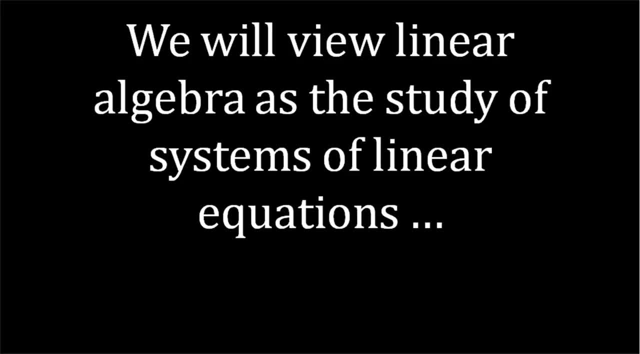 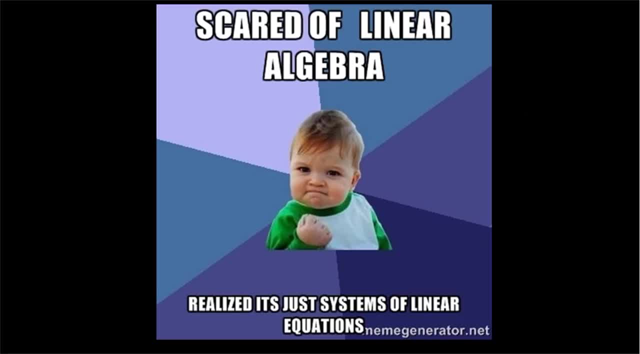 course for us. So here we go. We're going to view linear algebra as the study of systems of linear equations. Now I'm going to pause here so everybody can do kind of a fist pump, because linear equations is something that you are probably familiar with. You've probably solved small systems of equations. 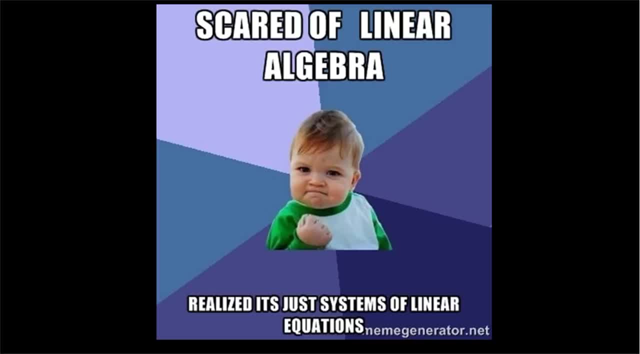 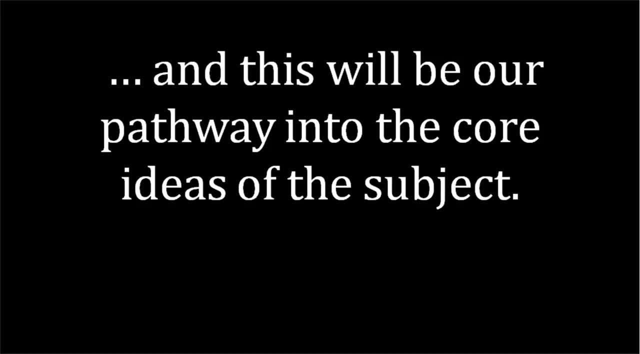 before in previous courses, whether it's pre-calculus or maybe even in calculus to a certain extent. So this is good. This is something that you are likely very familiar with, So this will be the pathway that we are going to take to explore the core ideas of this subject of linear. 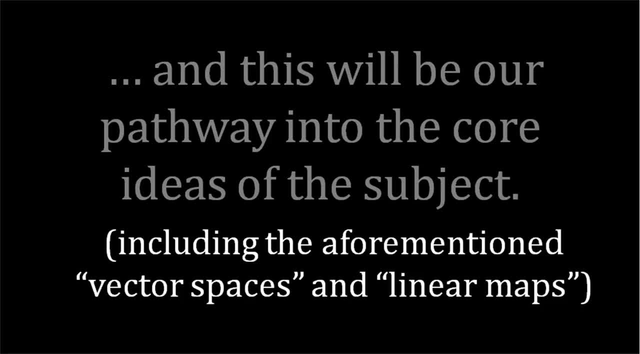 algebra, and along the way, we are going to come across these vector spaces and linear maps that were mentioned in the Wikipedia definition. So indeed, we are going to be learning about those things, but maybe it's not a great to start with those. So you might. 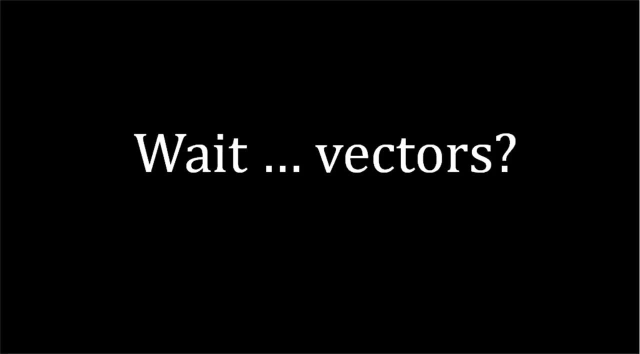 be saying: wait a minute. I thought that I knew how to solve systems of linear equations. What does vector, what do vectors have to do with anything? And so we're going to look at an example here and try to answer that question. So here we have an example, a very basic example, of a 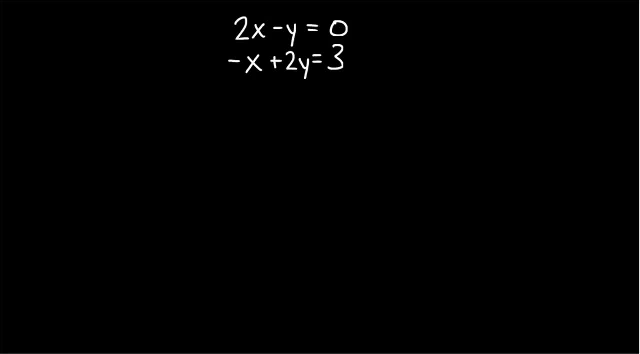 system of linear equations, and we're we're going to go about looking at it first the way that you are most likely used to, So that is, we're going to look at it by rows. In other words, we are going to consider these as well, the equations of lines, and we're going to graph these lines and the solution. 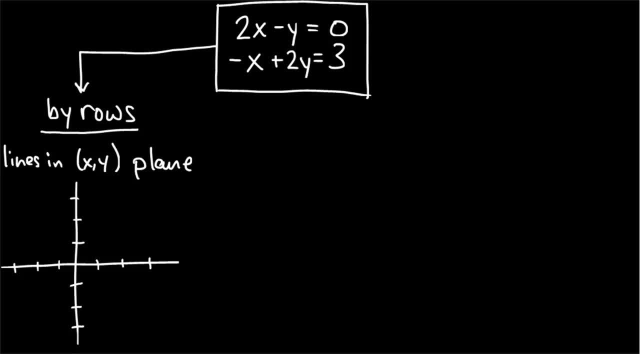 to the system, In other words, the. the point x, y that satisfies both of these equations is going to be our solution to the system. So we're going to look at it by rows and we're going to consider these as well- the equations of lines, and we're going to consider these as well the solution to the system. So we're going to 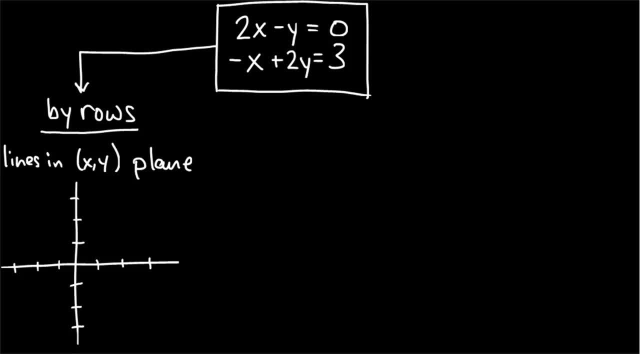 be the intersection of the two lines. So we can start by graphing these lines by a fairly familiar method, I'd say by finding the x-intercepts. So the x-intercept of the top equation is the origin, and the other one you can do a little algebra behind the scenes and find out that it's minus. 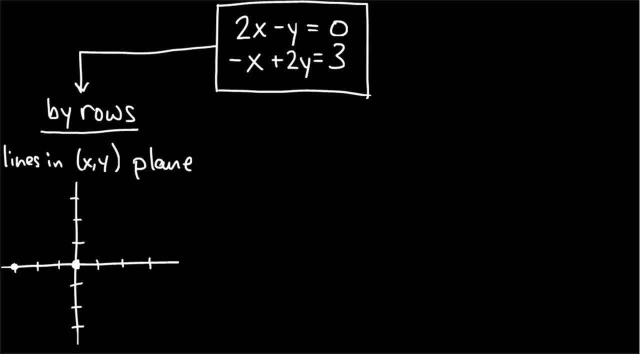 three zero, And then we can use what we know about slope to plot other points on these lines and graph them, And you can see that this was carefully chosen so that everything would work out nicely. We see that the point of intersection, in other words the solution to this, 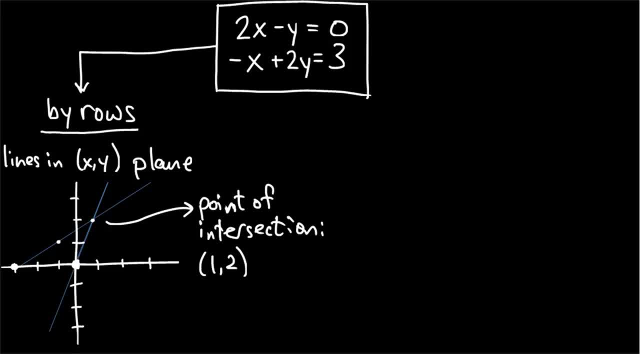 system, the point that satisfies both equations is one two. So that's, that's the relatively familiar way to do it. There are other ways to solve it. you can solve it by substitution or something like that, but this, I imagine, is a fairly familiar way. Let's take a look now at a way that is probably. 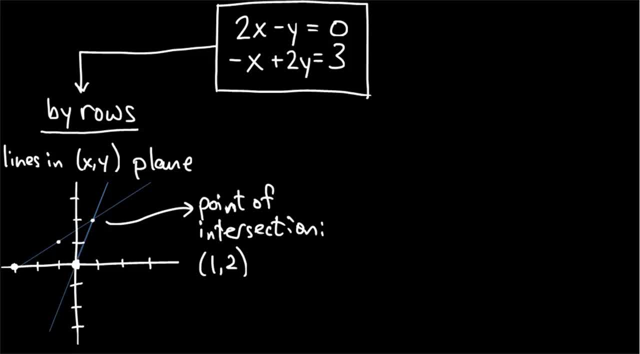 unfamiliar but is going to help us out. So let's take a look at a way that is probably unfamiliar but is going to provide us with lots and lots of valuable information. So we're going to look at this by columns. This system of equations we can see is equivalent to this vector equation that I've 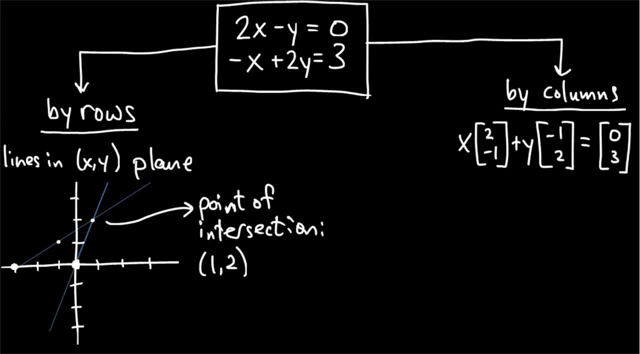 written over here on the right hand side. So there's a little bit of a different focus here on the left hand side. when we're looking at it by rows, the solution to the system was the point of intersection of these two lines, But here basically it's asking for a linear equation. 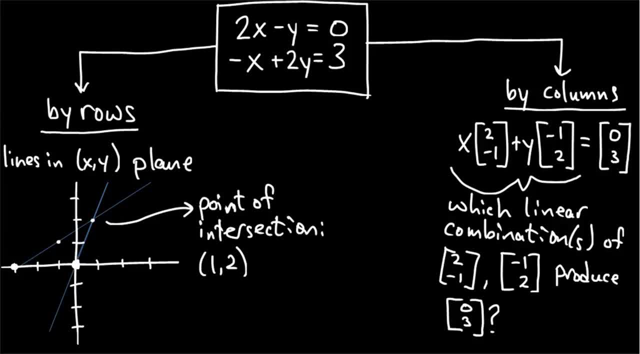 So what are the linear combinations of the vectors 2 minus 1 and minus 1, 2 that will give 0, 3 on the other side. So which linear combinations of 2 minus 1 and minus 1, 2 produce the vector 0, 3.. So of 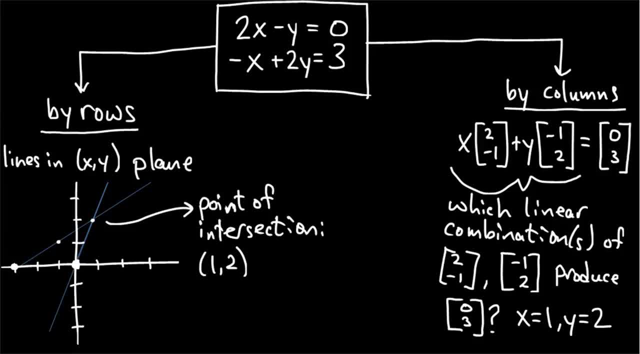 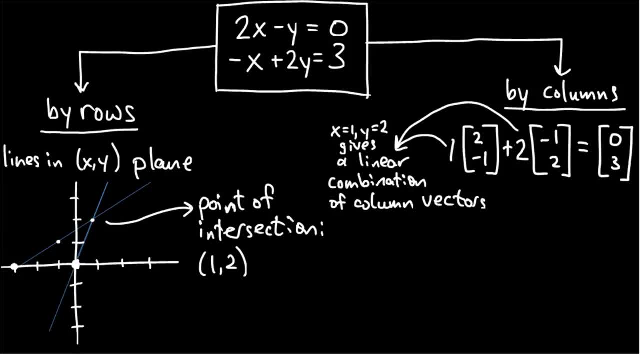 course we know. we already know the answer to this because we did the. we did it by rows first. So we already know that x equals 1 and y equals 2 are going to give us the solution here. So if we plug this in, you can use vector arithmetic to verify that this is indeed a solution. So again there they. 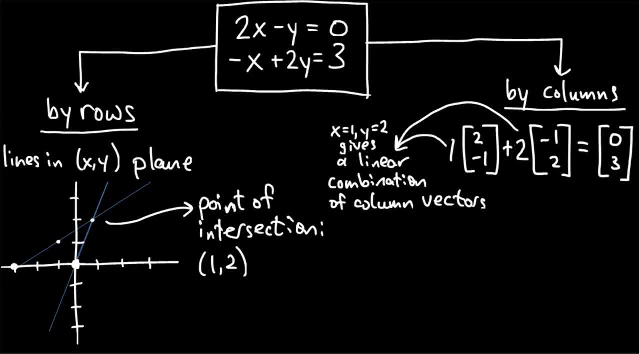 are identical ways of solving the problem. They're equivalent ways, I should say, but from drastically different viewpoints. So over here again, it's the point of intersection, and over here, 1 comma 2 is a linear combination of these what might be called column vectors. So we drew, we drew a nice picture. 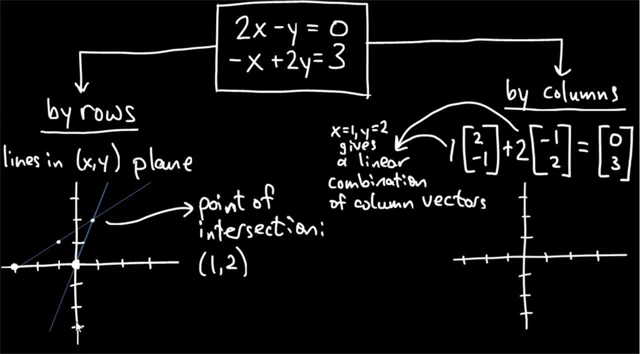 here. So let's go ahead and do the same, just to just to get a different viewpoint on this. So if we graph the vectors, If we graph this vector equation, you can see that first we depart from the origin and this takes us to 2 minus 1, and then it says: well, we want two copies, we want to add two copies.